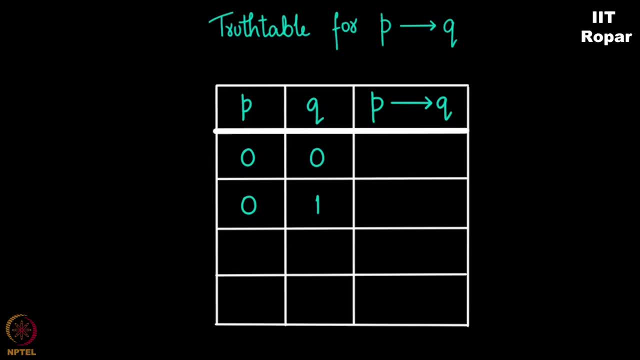 Let us start P Q. P is 0.. Q is 0. 0, 1. 1, 0. 0. 0. 0. 0 is P, implies Q-Always see this as P is a smaller set. 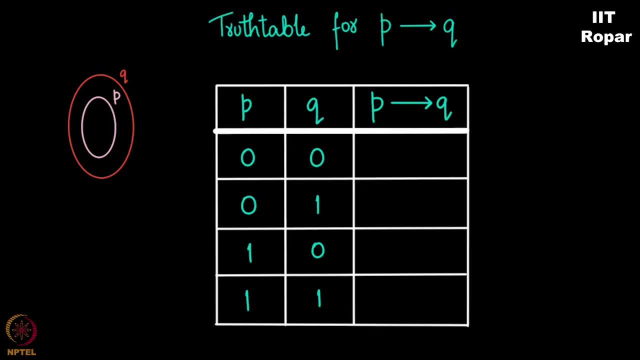 Q is a bigger set, like the New York and US example. Whenever you say P, some statement is true, you infer that Q is also true. This P implies Q, and New York and US doesn't seem to be the same, but you will soon realize. 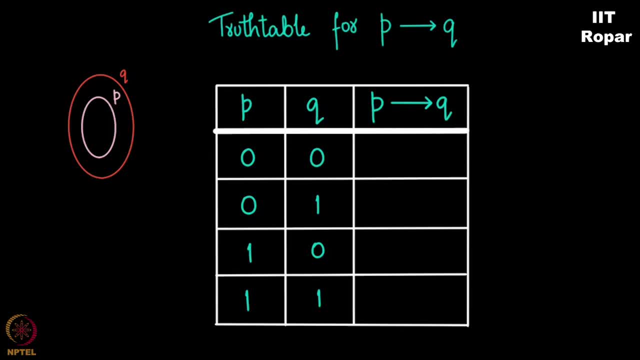 they are the same. Let's see how. When something is not in P, can you conclude include that something is not in Q? is what we are asking here. Do you think when P is 0, Q is 0? Stated differently? all I am asking is: can it so happen that inside this set there is 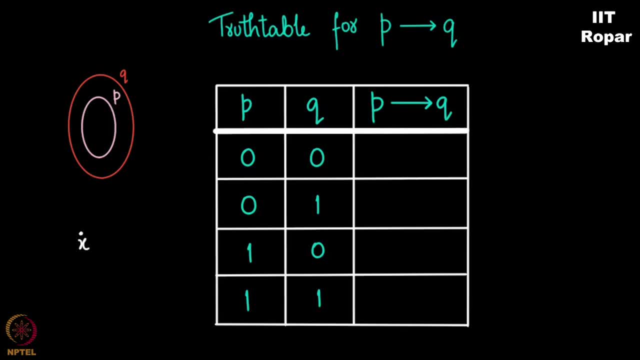 no element Given an element X, which probably is in the universal set. forget about A and B. A is a smaller set, B is a bigger set containing A and there is a universal set, U. If I give you an element X and that element is not in A, can you say that that element is not in? 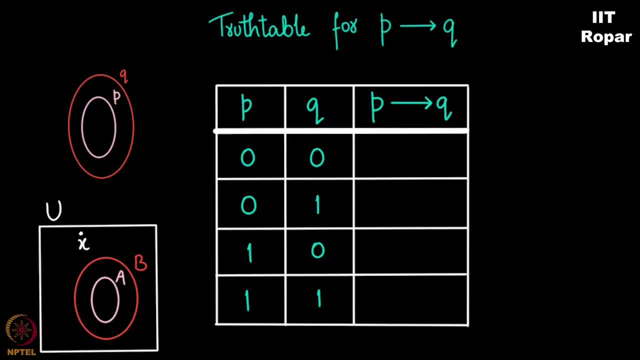 B. Not necessary, but yes, can be true. Look at this statement: When something is not in A, it could be in B, but not necessary, is all I am saying. Now look what is the next statement. An element is not in A. can it be in B? 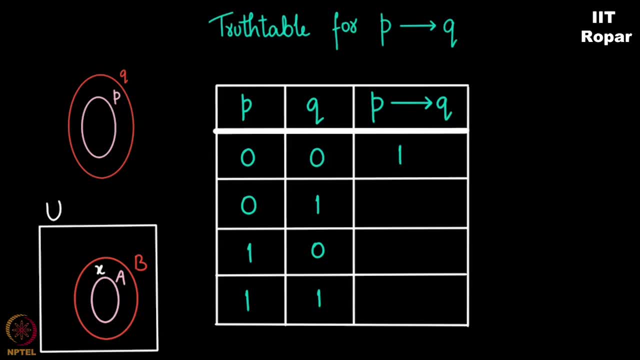 Not necessarily, but yes, it can be true. Same statement. You see Now what is the next statement: One and zero. An element is in A but not in B. Is that possible? That is impossible. First one is not necessarily true, but yes, can be true. 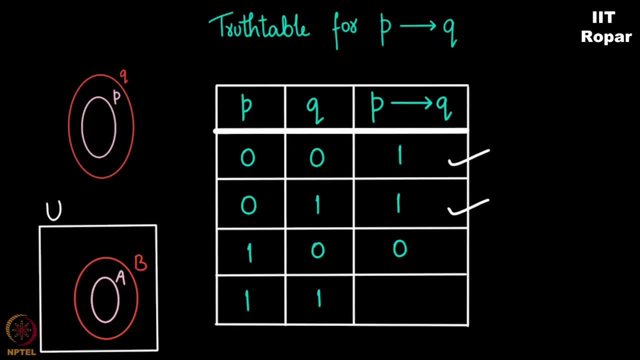 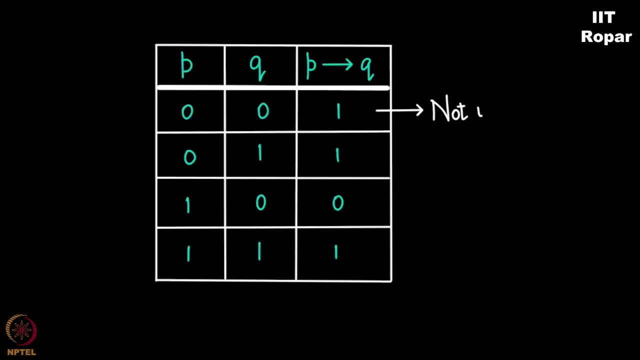 Second one is also not necessarily true, but can be possible at times. Third one is impossible. Fourth one is: an element is in A implies the element is in B, also Very true. This is always possible action. You see, first one is not impossible. 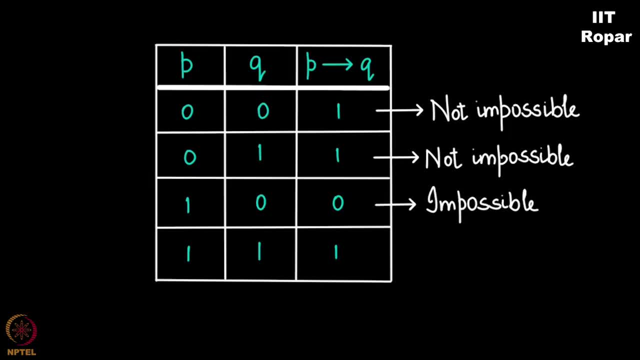 Second, one is not impossible. Third, one is impossible. and fourth one is: let us put it under the not impossible category, Correct Now. when it is not impossible, we write one. When it is not impossible- always possible, we write one. When it is impossible, we write zero.